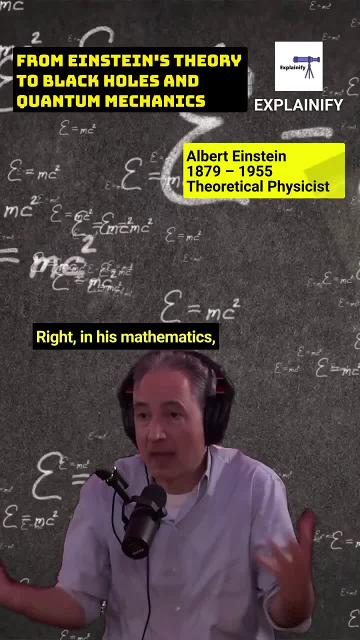 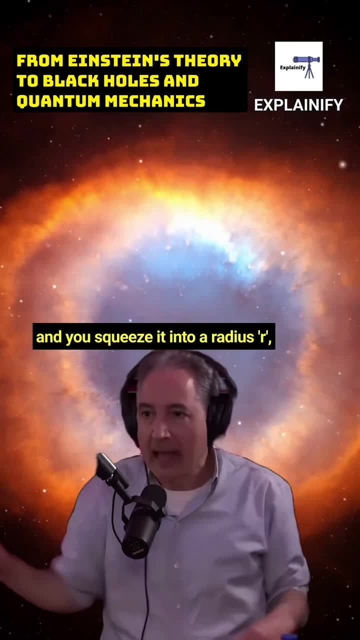 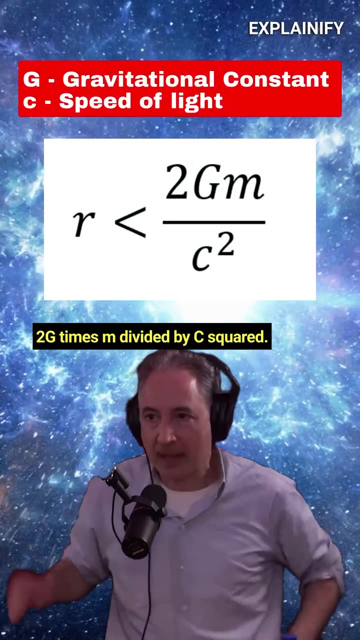 You look at Einstein's equations, right in his mathematics There's a little formula that you can see where it says: if you have any mass m, whatever mass you want, and you squeeze it into a radius r that's less than two times Newton's constant, 2g times m divided by c squared speed. 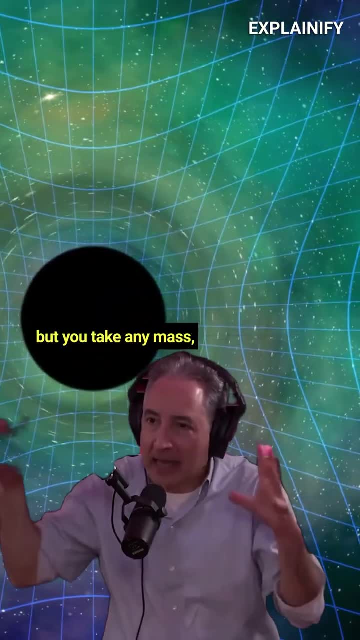 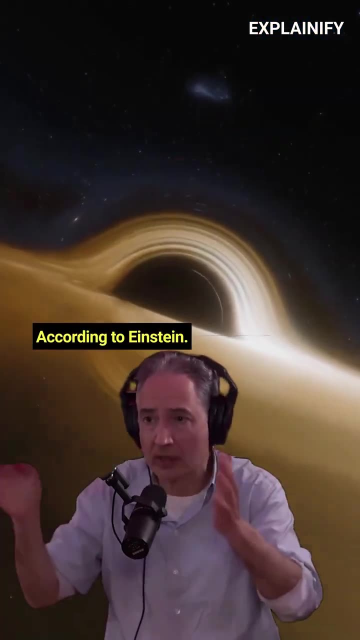 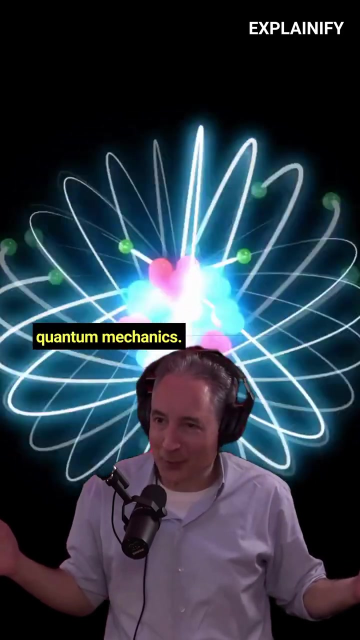 of light squared A formula. Details don't matter, But you take any mass. if the radius within which that mass sits is less than 2gm over c squared, it is a black hole and a story according to Einstein. Now, Einstein left out quantum mechanics, Weirdly right, Because his Nobel Prize was for quantum. 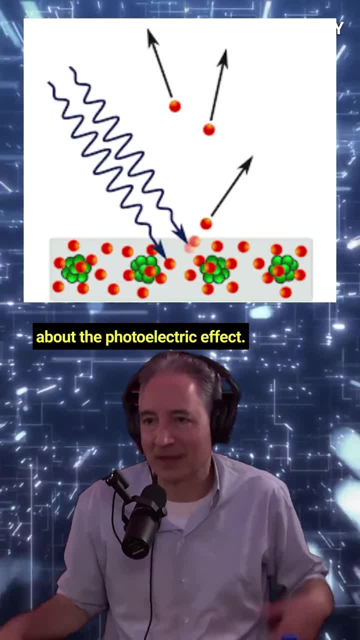 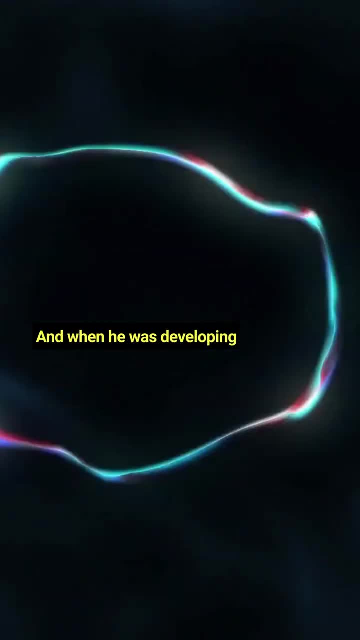 mechanics. It was for a paper he wrote in 1905 about the photoelectric effect, But he never really believed that quantum mechanics was the true description of the world, And when he was developing the general theory of relativity he was just thinking about. 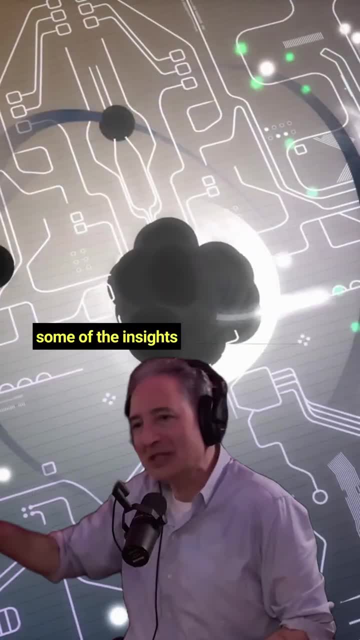 gravity and not quantum mechanics, And so people are using some of the insights from quantum computing to understand questions about black holes in space time. 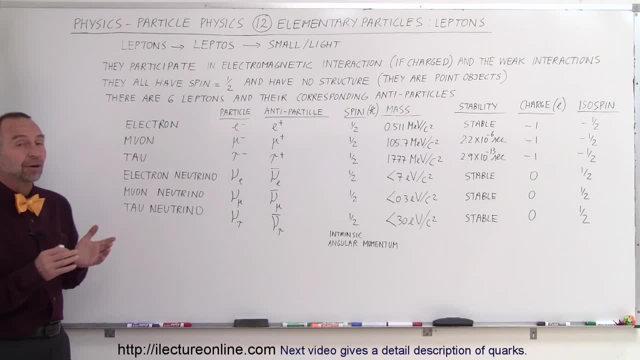 Welcome to ElectronLine, and now we're going to take a closer look at the elementary particles called leptons. So we know that there are six leptons, and here they are. There's the electron, the muon, the tau and then the three corresponding neutrinos. Now let's look at 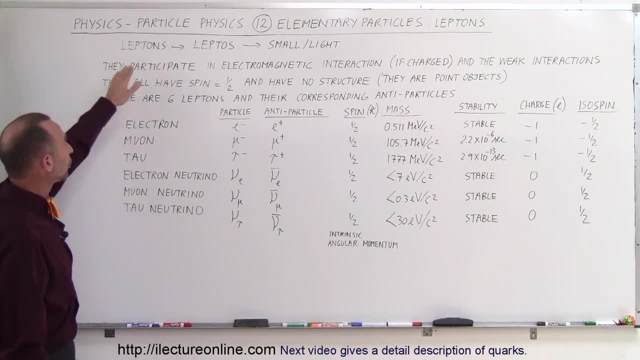 some basic properties of leptons. So leptons come from the Greek word leptos. that means small or light, So leptons tend to be very small particles. There's one exception though: the tau is not so small. We'll get into that in just a little while. But for the ones like the electron and the 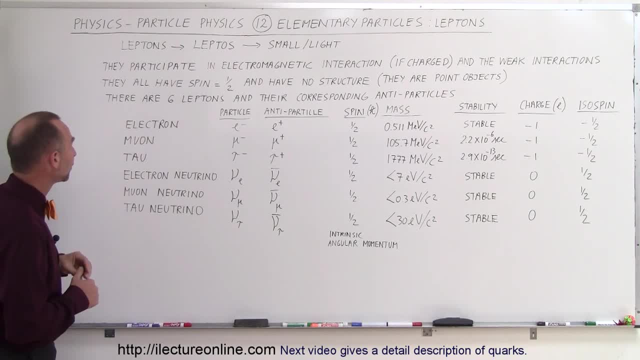 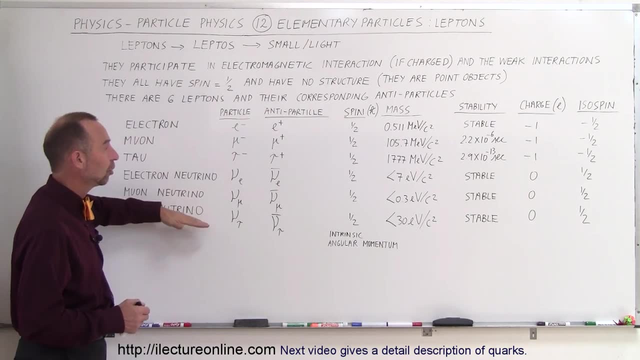 neutrinos are very tiny particles in relation to other particles, So they participate in the electromagnetic interaction. if they are charged Now, the neutrinos do not carry a charge. You can see here: the charge is zero for the neutrinos, so therefore there's no electromagnetic interaction.